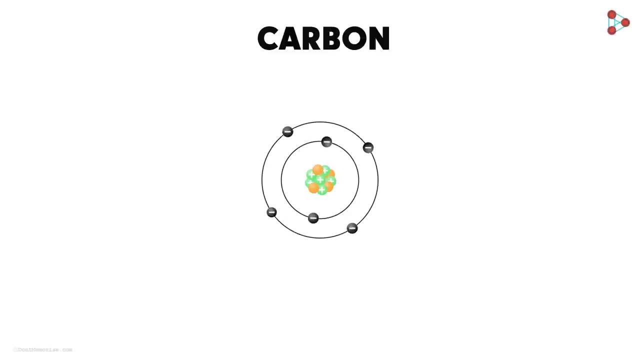 like this. Yes, The electronic configuration of carbon is 2-4. That means it can either donate or accept four electrons to achieve stable state. However, it's not as easy as it seems. This is because donating the four electrons will mean that the atom is. 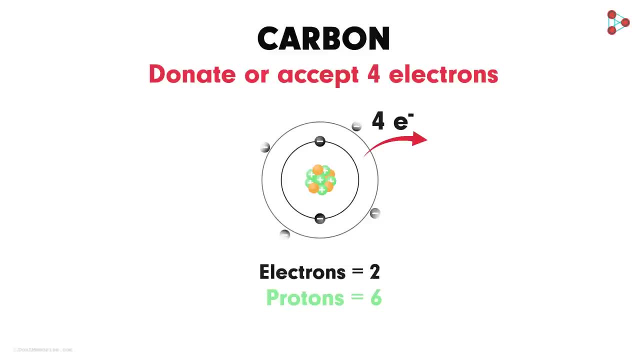 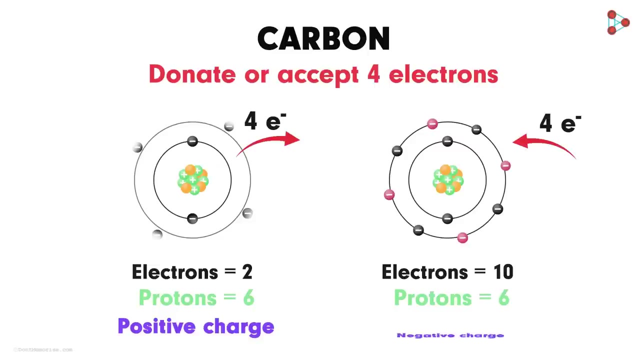 now left with only two electrons, But the number of protons still remain the same. right. That means the atom will gain positive charge and will still be unstable. Similarly, accepting four electrons will also lead to a situation where the carbon atom becomes negatively charged. 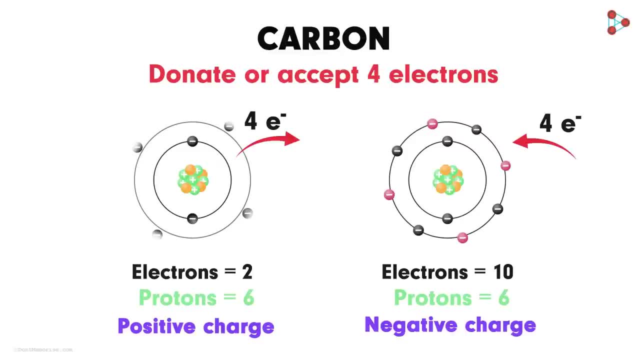 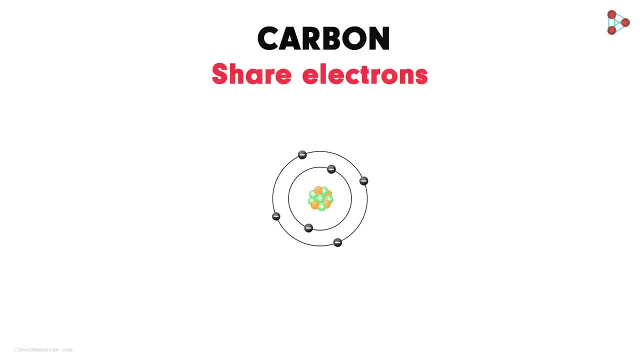 Thus, both the situations would lead to instability of the carbon atom. So the option that carbon adopts is to share electrons. Sharing in carbon can take place up to four electrons. That means carbon can share all its valence electrons with any other atom. We know that such sharing 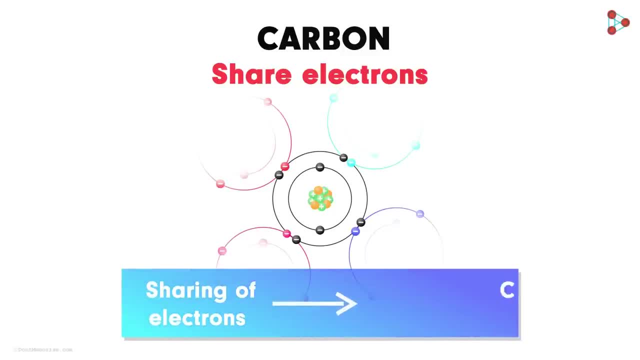 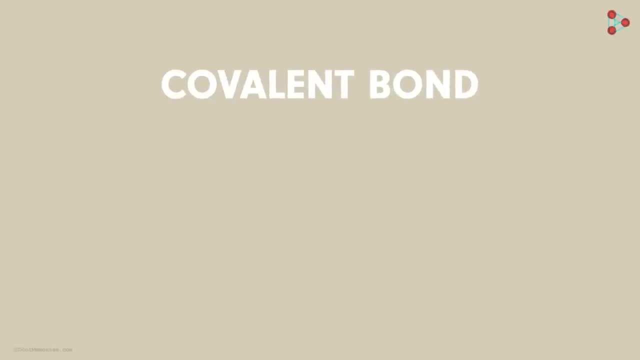 of electrons leads to a special type of bond formation called the covalent bond. So to understand carbon chemistry, we need to understand covalence. How can we define a covalent bond? by the way, In simple words, it's the bond formed. 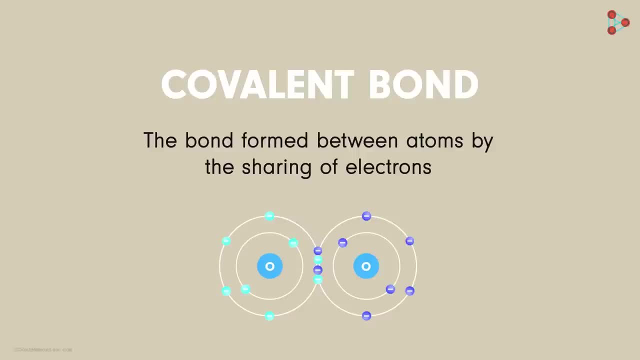 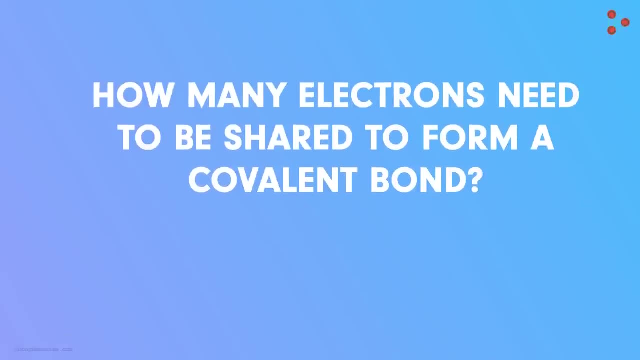 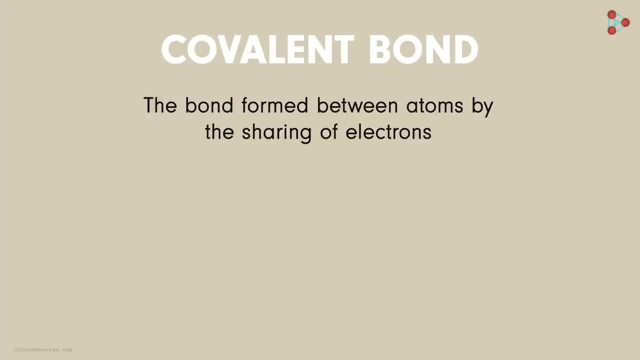 between atoms by the sharing of electrons. Now the next question that pops up in our mind is how many electrons need to be shared to form a covalent bond. Is it one electron or a pair, Or more than a pair? Can you guess? Let me help you with the answer. When we say: 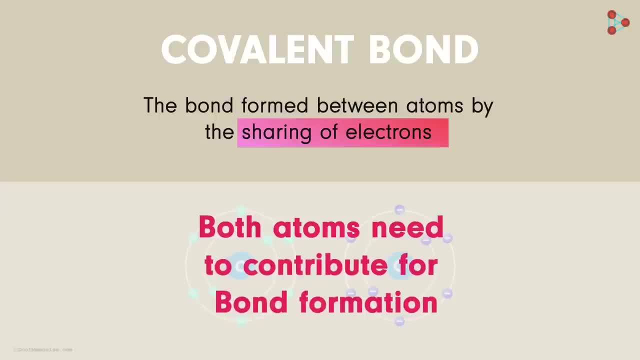 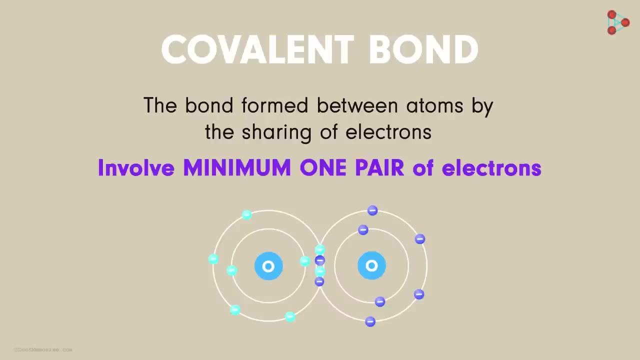 sharing. it means that both the atoms need to contribute for the bond formation. right, It indicates that each atom will give at least one electron from its valence shell. Does that tell us that a covalent bond will involve minimum of one pair of electrons? Yes, a covalent bond needs at least two electrons, or simply. 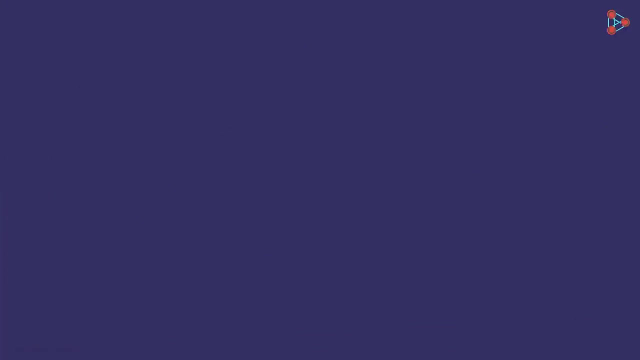 one pair of electrons. Such a type of covalent bond, where one pair of electrons is shared between the atoms, is called a single covalent bond. It is denoted by this term in order to find the covalent bond and its covalent bonds. 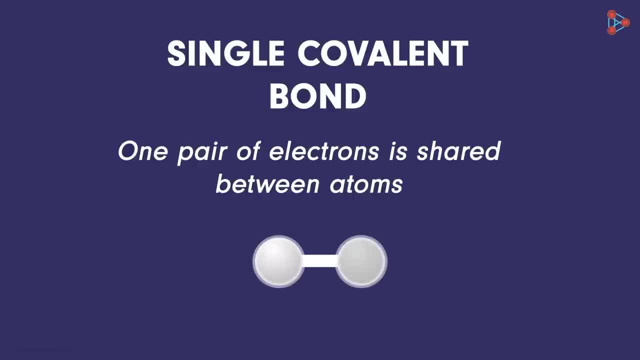 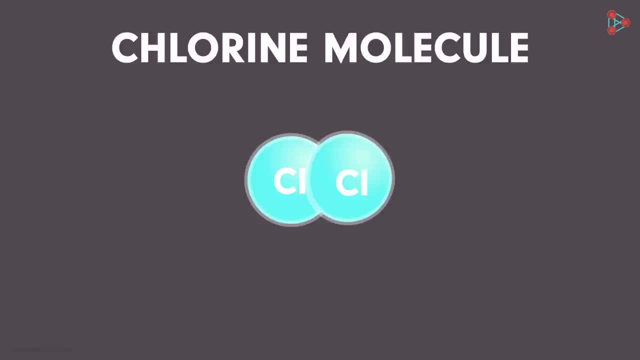 it by drawing a single line between the two atoms. A simple example that explains this type is the formation of a chlorine molecule. How do you think this molecule was formed? We know that chlorine has seven electrons in its outermost shell. That means only one electron is needed by it to 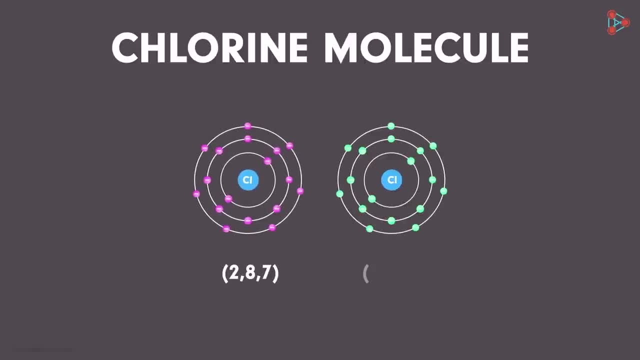 complete the octet. Now here's another chlorine atom which again has seven electrons in its outermost shell. Both of them want one electron each, And that is why we find two chlorine atoms coming together and forming a bond by sharing one electron pair. 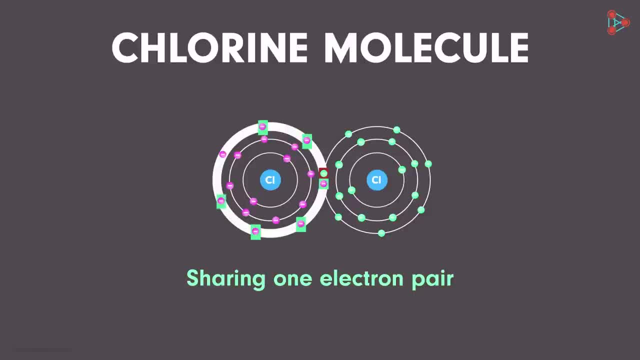 Now, if we look at this orbit individually, it has eight electrons, And this orbit, too, has eight electrons. Stability achieved for the chlorine molecules. This was an example of a single covalent bond. So do all atoms form covalent bonds by sharing a. 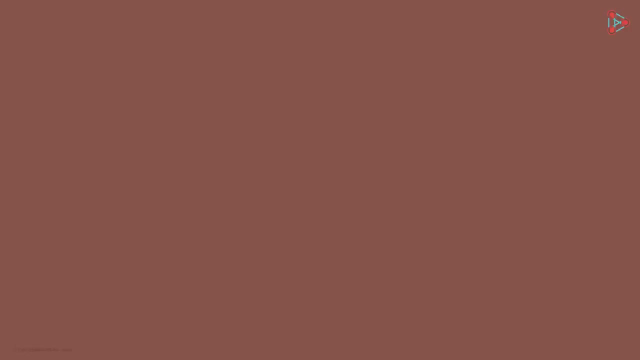 single pair of electrons. Think for a moment. We know that oxygen is in the diatomic state. That means one oxygen atom forms a bond with other oxygen atom to form a stable molecule. Do you know how many electrons are shared in this bond? 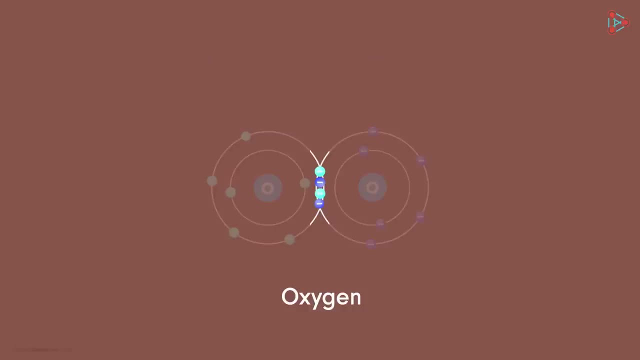 What do you notice? There are four electrons shared. That means both the oxygen atoms contribute two electrons each, thus giving two pairs of electrons in the bond formation. So is this not an example of covalent bond? Well, it is, But covalent bond has one pair of electrons being shared, right? 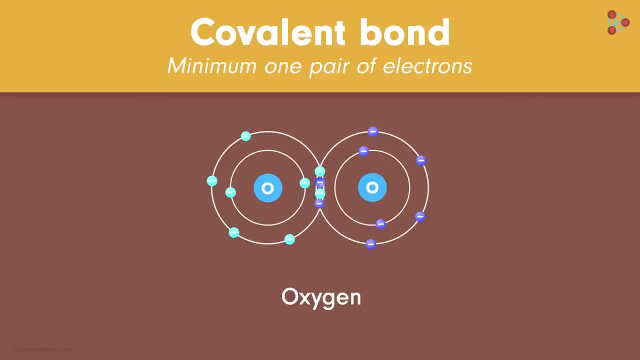 Don't forget, it is a minimum of one pair that's needed for formation of the covalent bond. That means this case is also an example of a covalent bond. Such a covalent bond, which involves two pairs of electrons getting shared, is called a double. 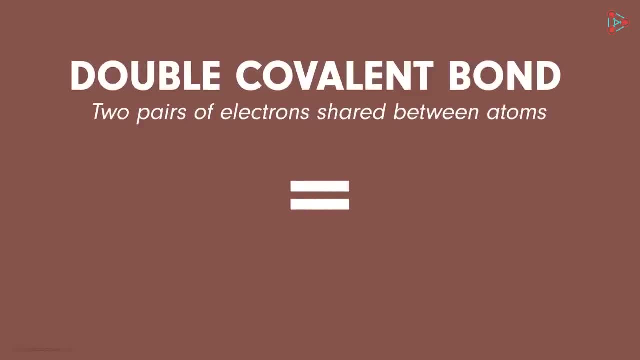 covalent bond. It is represented by two lines written between the two atoms. That is why it is called a double covalent bond atoms, Just like this, as seen in case of Oxygen. Now on the similar lines. can you give me an example where more than two pairs of electrons